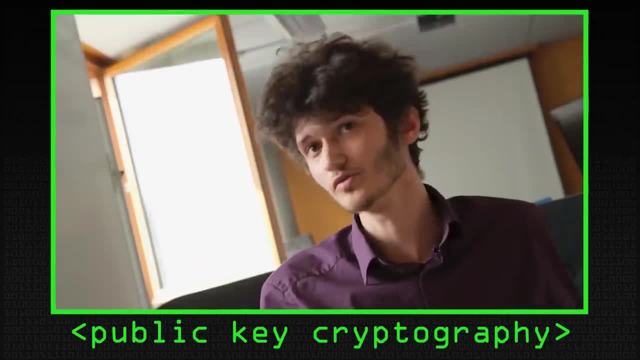 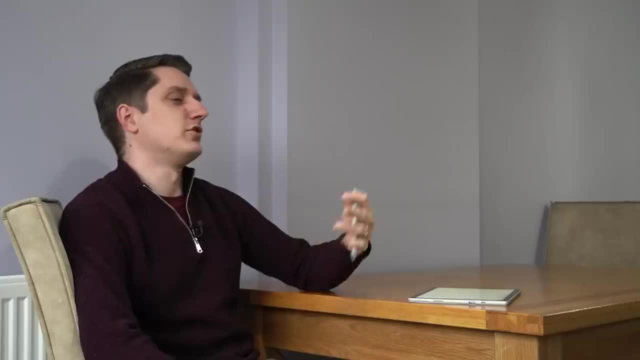 and you should definitely, you know, check that out. So, if you recall, in public key you have a public key and you have a private key and they're kind of the inverse of one another, so you can encrypt with one and decrypt the other one, So I can, for example, if you have a public key, I can. 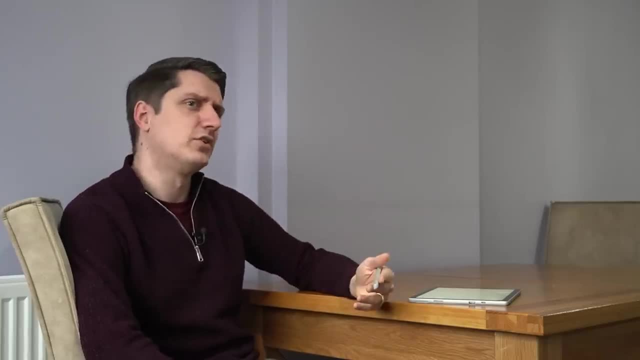 encrypt something with it and send it to you, But actually we don't tend to do that. very often We could do that, but encryption with something like RSA is not that quick and, for very long messages, becomes a little bit impractical. There are other reasons as well in terms of the fact. 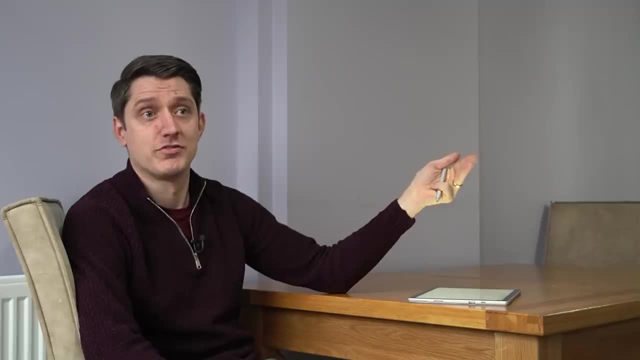 that we use these keys for a very long time and people prefer to rotate keys more often. So these days for actual encryption, what we would tend to do is just encrypt things using something like AES and symmetric keys. So you use this kind of thing to verify who you. 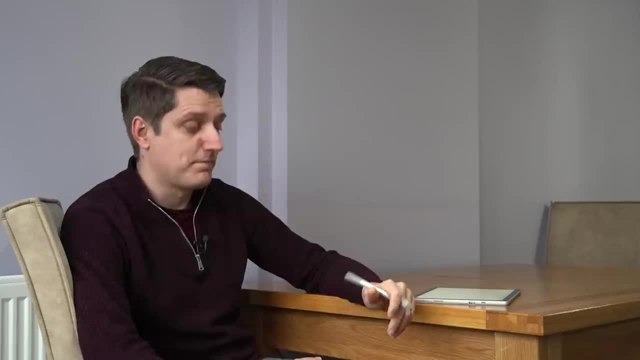 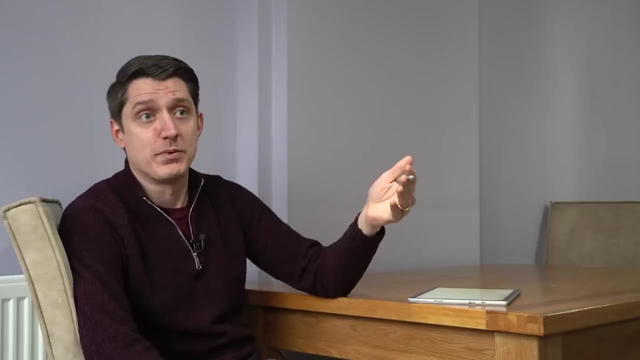 want to encrypt And then move on and establish something else. Yeah, that's exactly right. The way that we use something like RSA or the other signature schemes is going to be that we verify the identity of one of the people in the conversation and then 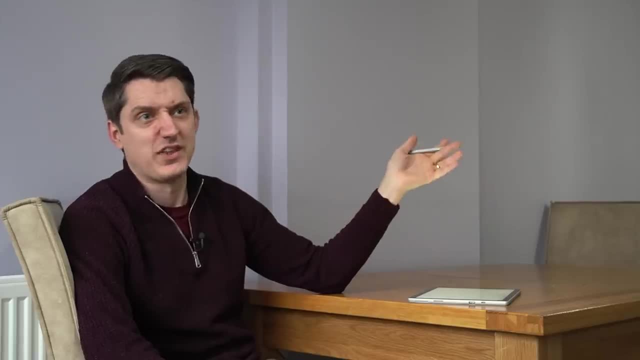 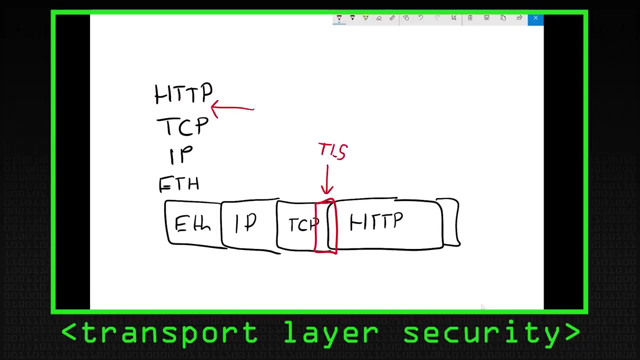 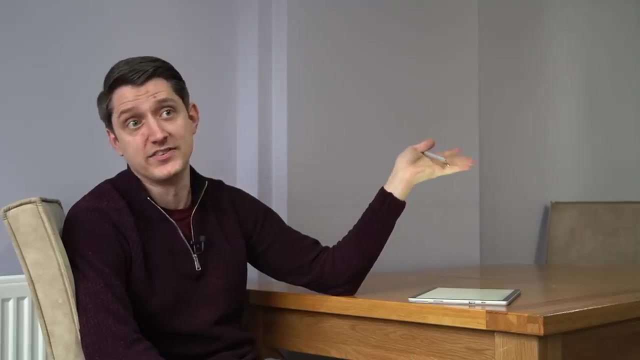 we revert to regular symmetric cryptography And we'll have done a key exchange or something like this. I mean, we talked about this in the TLS video, So part of TLS is a certificate and a digital signature and it only forms a part of the handshake, after which we just consider that done. 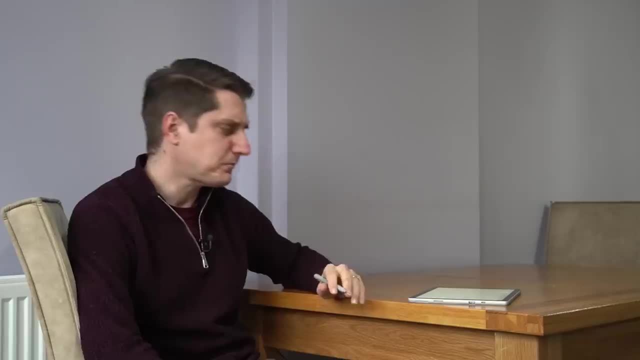 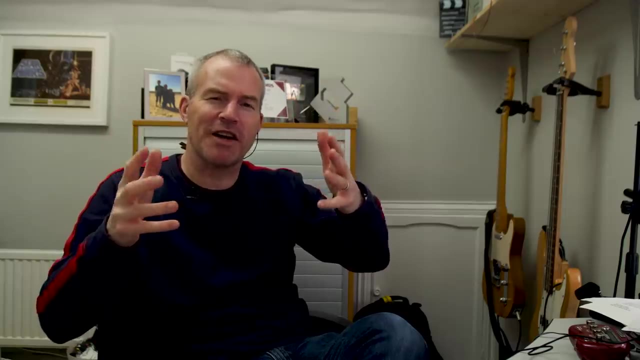 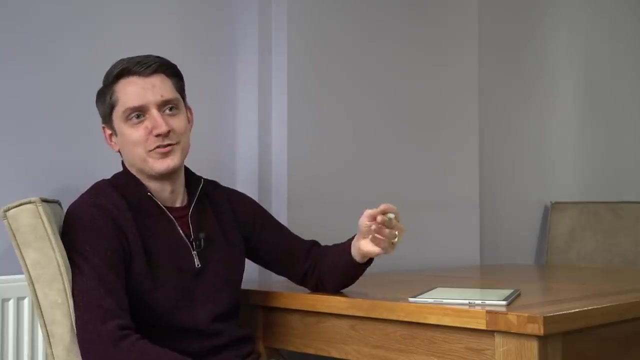 and then we move on. So what is a digital signature right? That's, I suppose, the first question In my head. I've got this idea of kind of like a bitmap 8-bit version of signing your name right. I mean, there are obviously lots of cryptographic things that we have to tick off right to make. 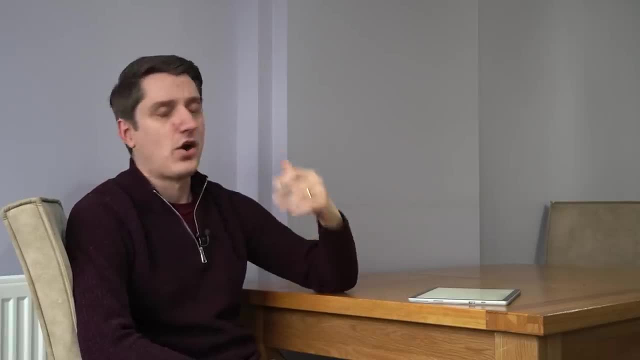 sure, it's not forgeable, But the idea is that I have a document or a message or something that I want to send you and I want to prove that it was me that sent it, And so to do that, I'm going to use my private key to sign a digital signature And basically what you're going to do on your end. 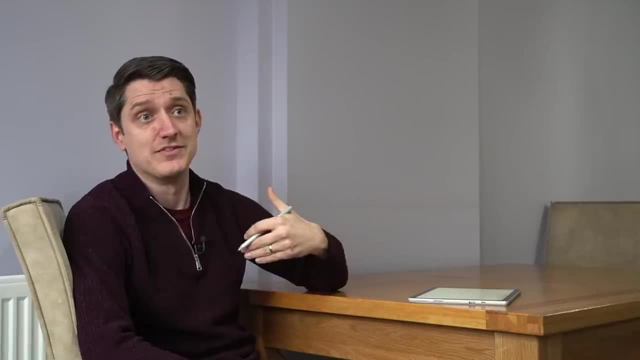 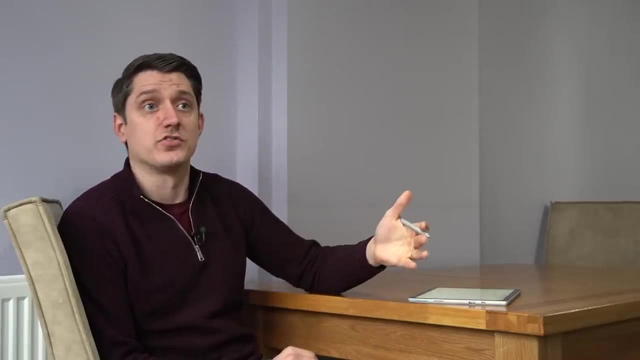 is: verify that signature and verify that it was actually me that encrypted it. That's the idea. So, when we perform this process, what we tend to think of is the person that's doing the signing and the person that's doing the verification. right Now, I, you know, I might nod to RSA, or. 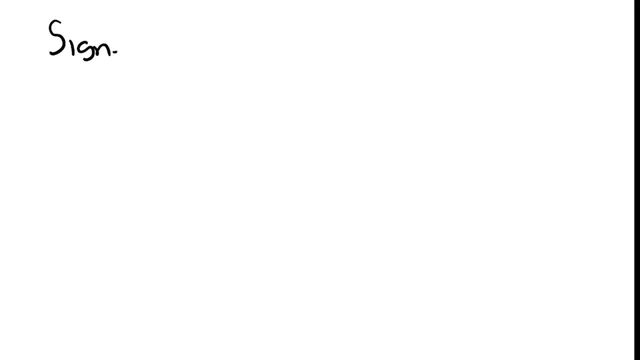 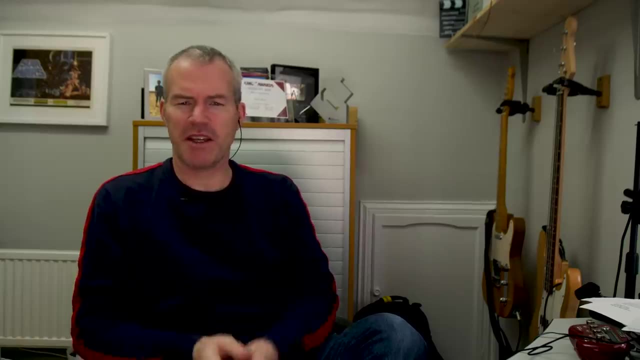 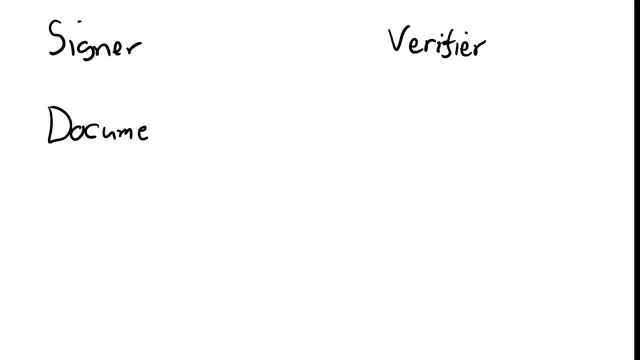 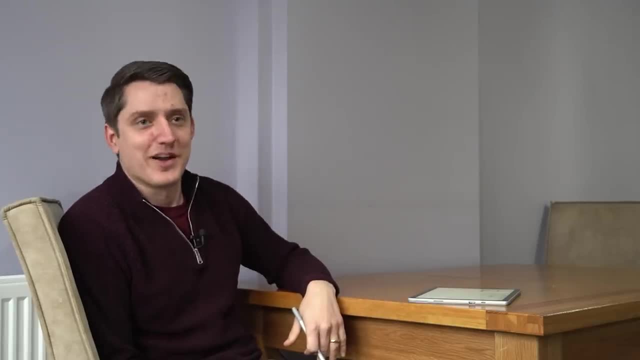 I don't know, I don't think. so, Yeah, okay, We've got some document or something like this or message. For now, let's not worry about how long it is or what. it is right, It could be a letter, It could be, you know, a mortgage application. It. 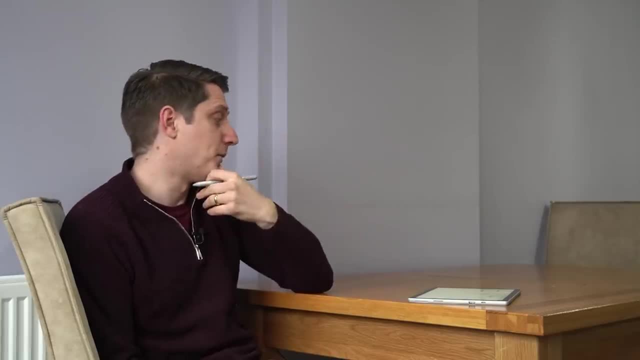 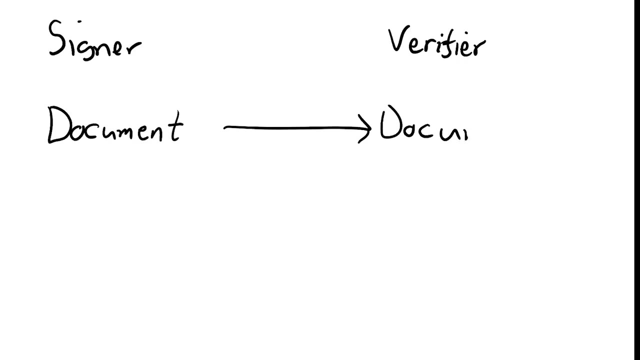 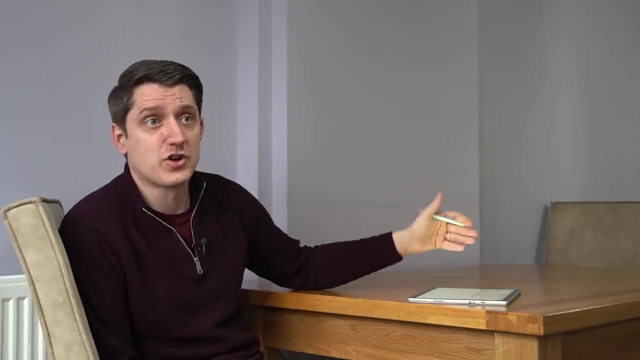 could just be part of a TLS handshake message. It's not really important. Now, this document is not currently encrypted and we're going to send it over to the verifier, like this, as part of our conversation. Now, the problem with that is it could be someone in the middle changing this document. 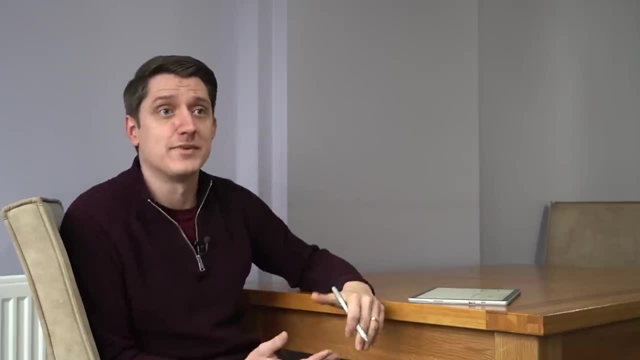 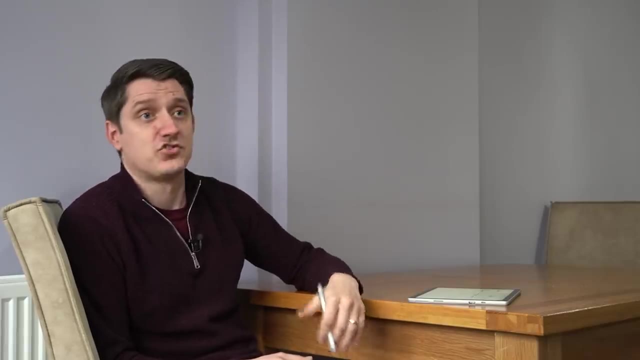 forging it. This could be a fake document. You know, we don't know that it's come from me. This is over the internet, and so when you send something over the internet, you can't guarantee that someone hasn't changed something or done something they shouldn't be doing. Now, if we had an encrypted 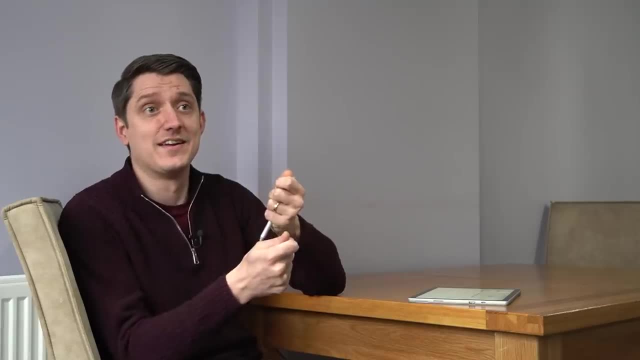 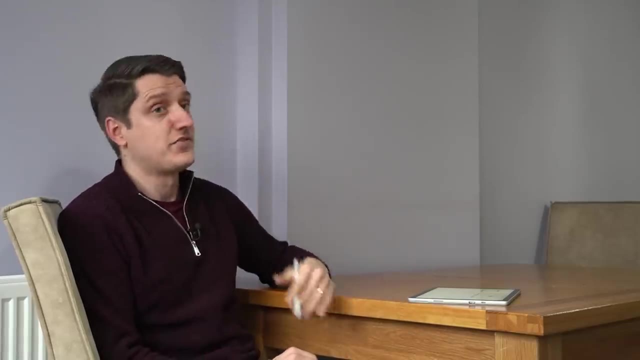 connection where we knew we had, we each had a key that would help. but we've still got the issue of how do you do this when you establish the key and during the initial handshake and things like this. So digital signatures form a big part of these kind of systems because, at the beginning at least, 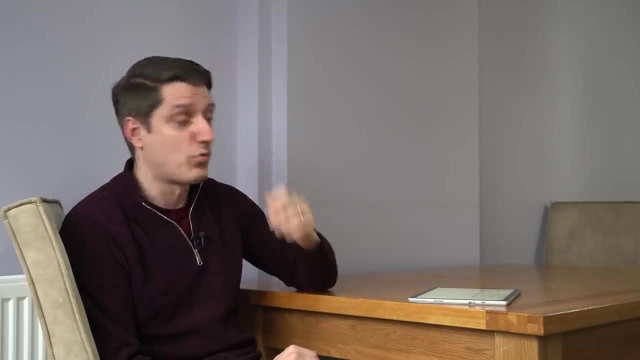 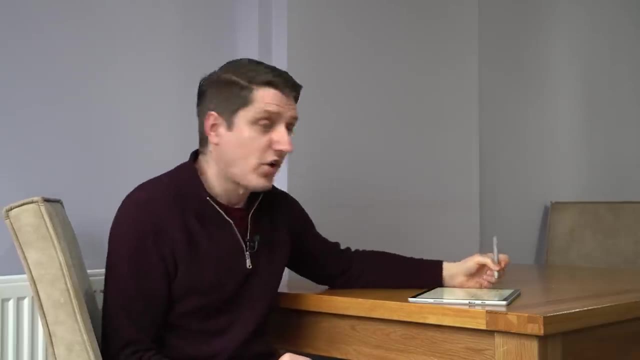 you're going to have to prove one of the identities At least, otherwise you're going to be finding no one knows who anyone else is, and that's going to be a huge problem. So what the signer is going to do is create a digital signature They're going to take. 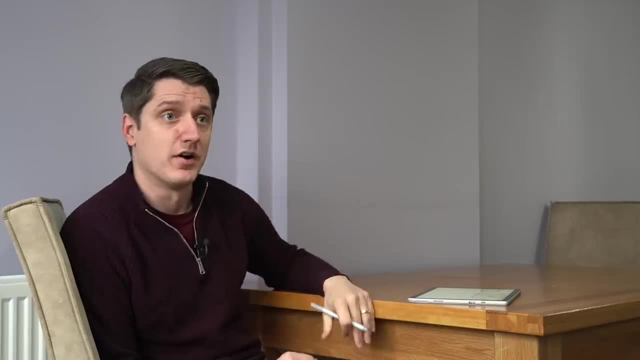 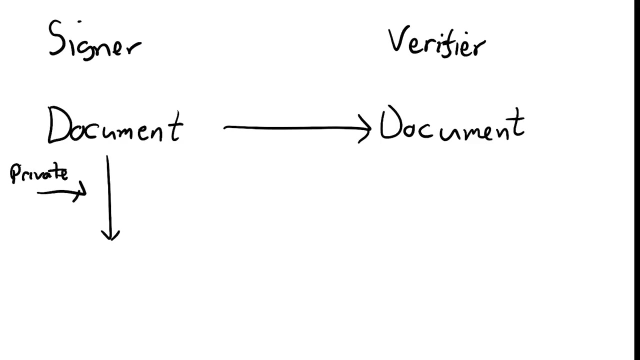 the document and we'll just simplify for a minute and then we'll build up a little bit of of sort of information in a while, right, and they're going to encrypt it with their private key. This is basically exactly like what Bob described, right? So this will form. 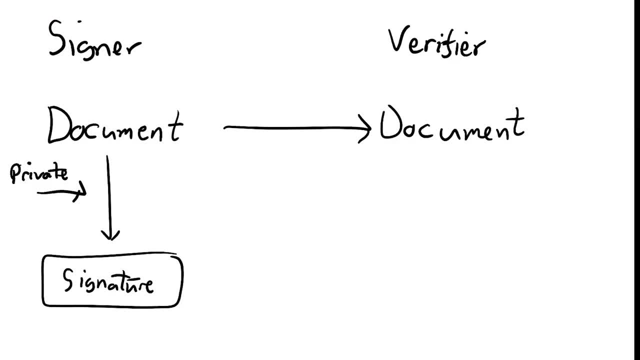 a signature. Now. they're the only ones that could have done that right, because they- only they're the only ones that have the private key right. otherwise, none of this works right. if they've got to do that way, they then send the signature over to the verifier right over the internet and the ver and the verifier can. 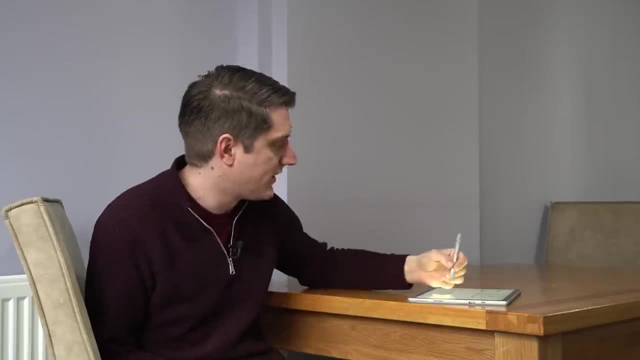 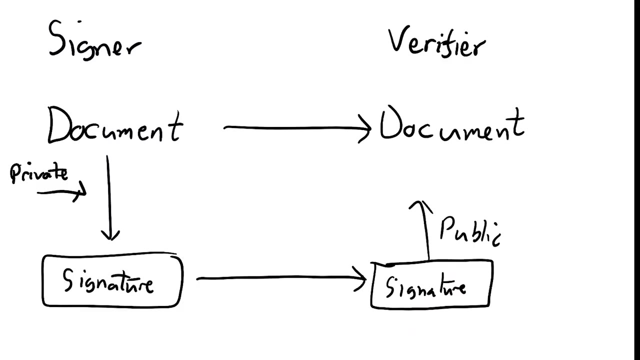 perform this verification process. so they can basically say, well, okay, what if we take this signature and we decrypt it with the public key? all right, so this is the signature here. what if we do take this and we decrypt it with the public key? because, remember, they reverse one another? 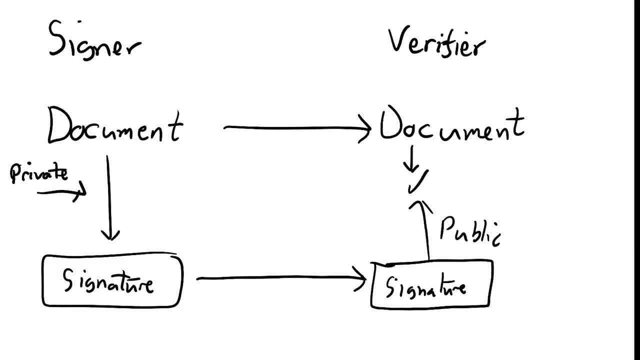 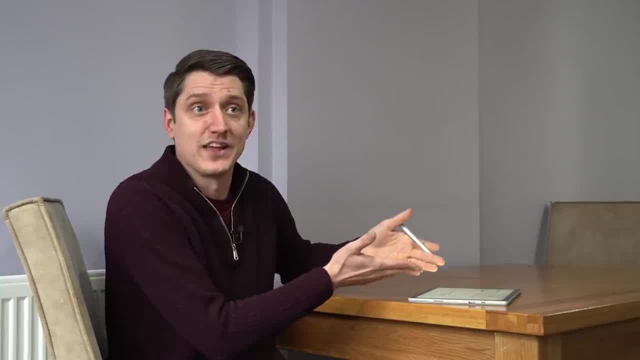 and then we can sort of work out whether the document and the signature match right, because if it was the original document that was encrypted using a private key, that original document is going to pop back out again, and then we can verify that that's actually taken place. if that's a big 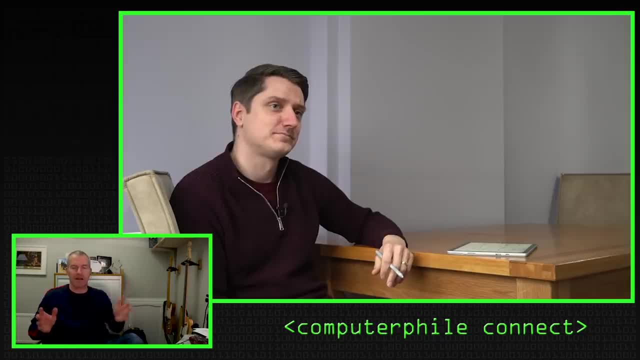 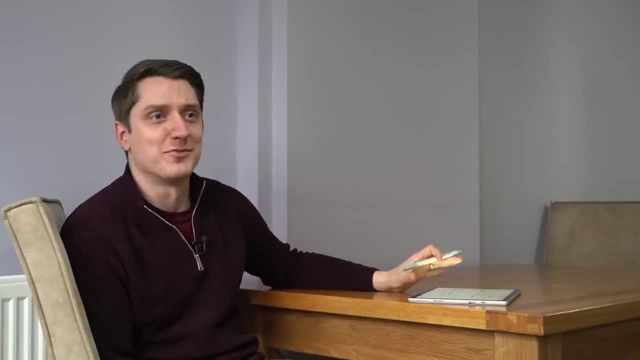 document. isn't this a bit wasteful, because you know, if it's gigabytes, like the video files that i might send, is that not a bit wasteful too? that's a huge problem, right, which is why i've oversimplified it, right, and everyone watching the video, who knows about this, is going to be like what when? 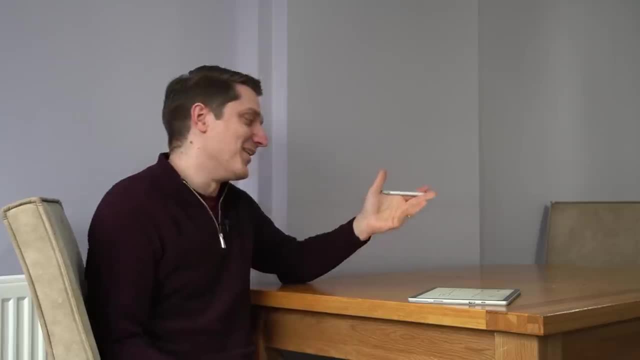 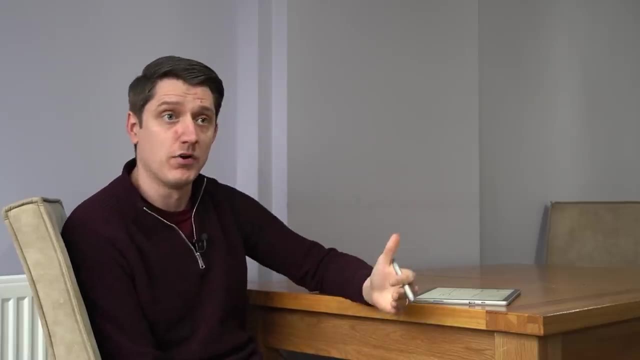 is he going to talk about hashing, right? well, now, now we're going to talk about hashing, um. this is- this is an oversimplification, because the problem is that this document could be any length, right, and it's a problem if it's very, very long, but it's also a problem if it's very, very short, right, if your document is literally the number one. 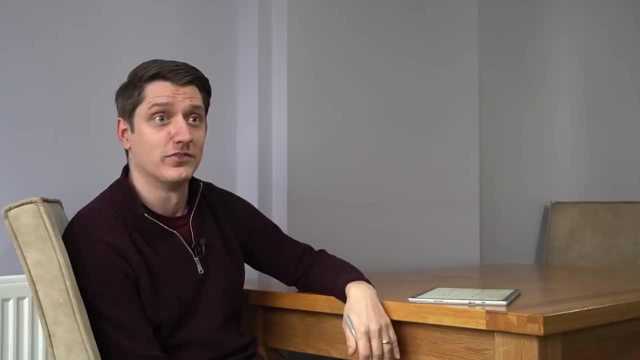 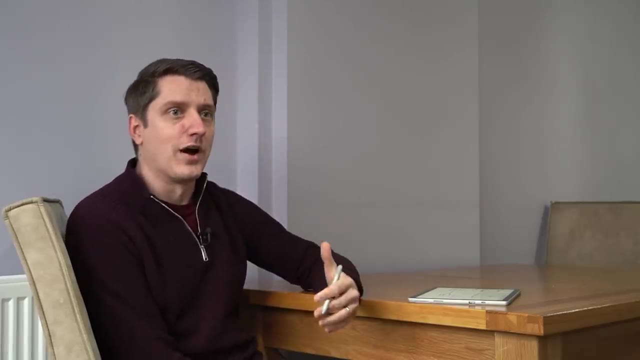 the encryption using rsa of that with any key is also one right, as a sort of contrived example right. so signature schemes like rsa don't work well when you have very, very short messages and we start to run into problems of computational efficiency and the fact that you're going to have to split the message up and sign multiple. 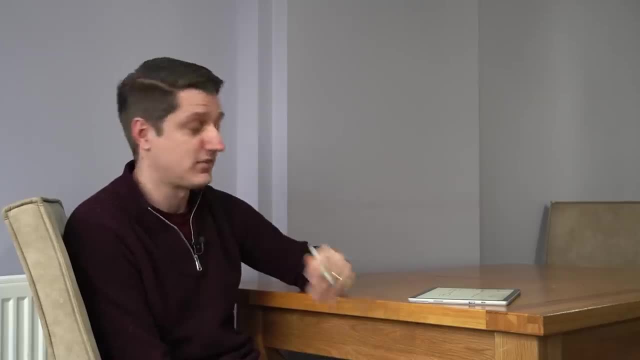 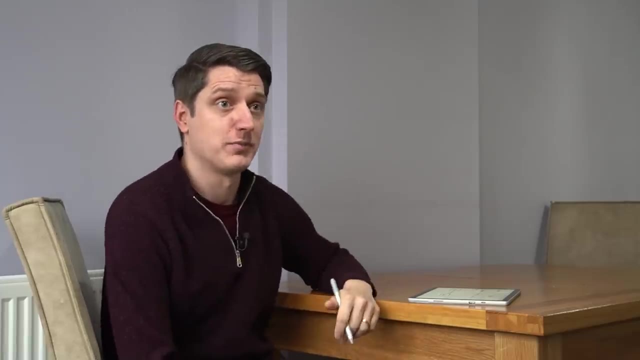 bits and then they can be reordered, and there's all kinds of attacks that you can run on this. so this isn't going to quite work, right? we want a scheme that will work however long the document is or however short the document is. so we're going to mix this up a bit, right? what we're going to do is: 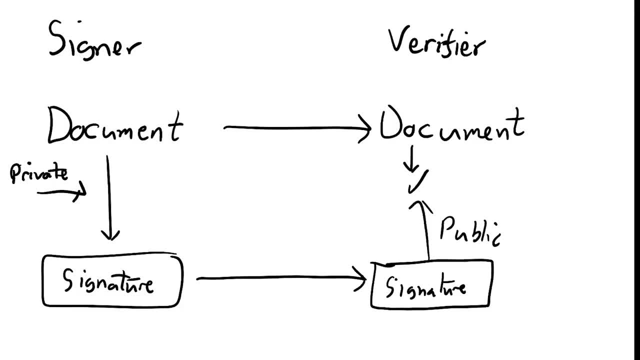 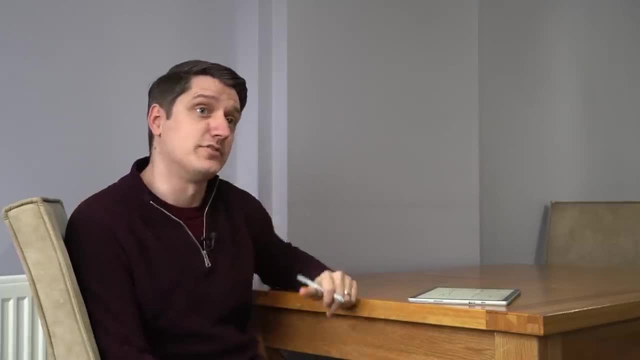 i'm going to change my pen color. it's all very exciting. we're going to insert a hash function here, so this is going to be a hash function. h right, and you know we might use something like this now that will take, as you know, any message length and turn it into a length of exactly 256. 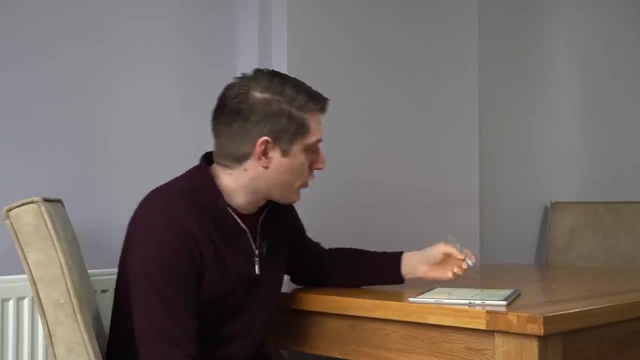 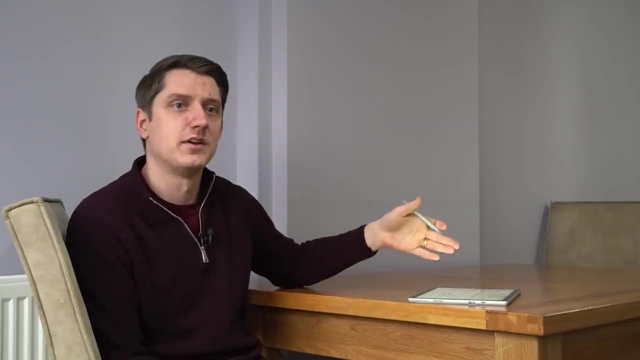 bits, which, for this purpose, is going to help us a lot. we're also probably going to want to add some padding, because typically 256 bits is quite short for this kind of signature scheme, so you'd usually sign a longer message than this. again, you don't know what the output of the hash is going to be if. 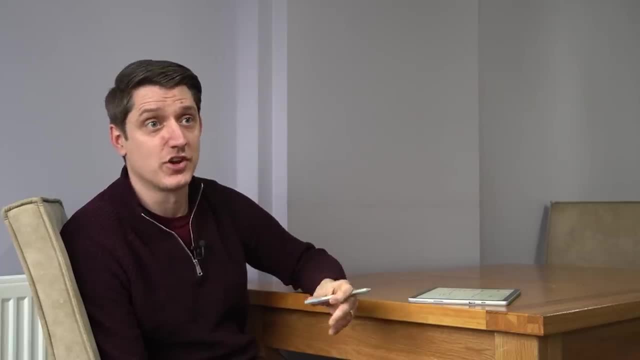 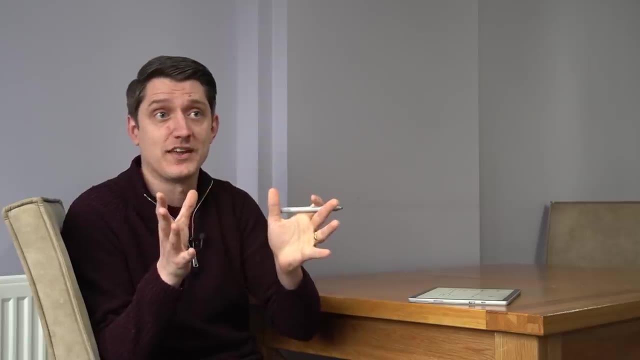 the hash ends up very, very small right, like in blockchain. that could be a security risk. we don't take that risk. so we're going to take the document and we summarize it using a hash function- maybe we add some padding or some other mechanism like this, and then we encrypt it using the private key. 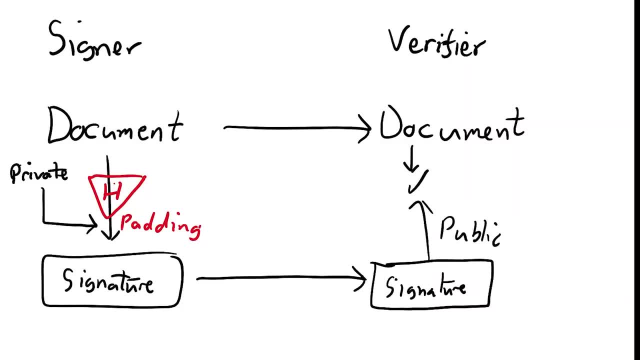 so this, this arrow here, goes away and we're going to take our private key and encrypt it there instead. so now the verifiers process has to change slightly to basically to match. so we're going to take the document and we're going to hash it, and then we're going to possibly add some padding. 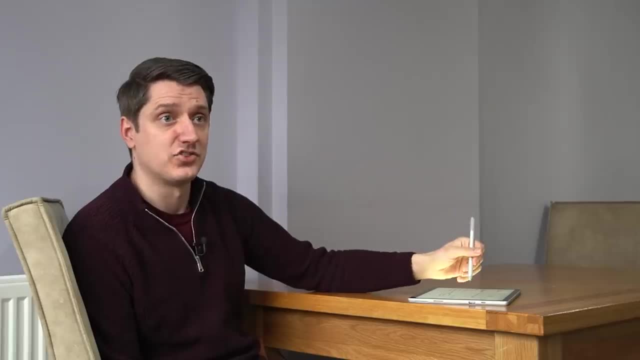 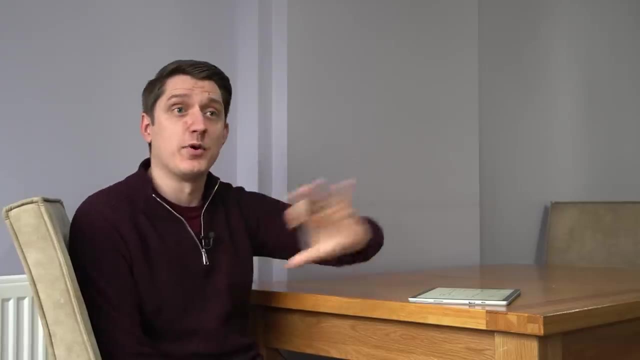 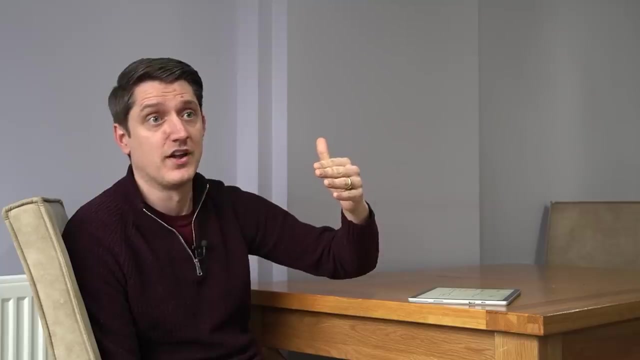 and perform the exact same process and we can work out whether that is going to match the one that's been decrypted using the public key. what we will normally do is ship these both off together in a conversation, so as, as an example, in tls, you will send a bunch of messages to each other and then at some point you will send a. 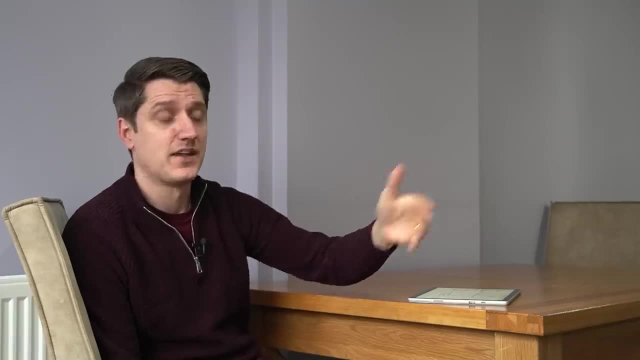 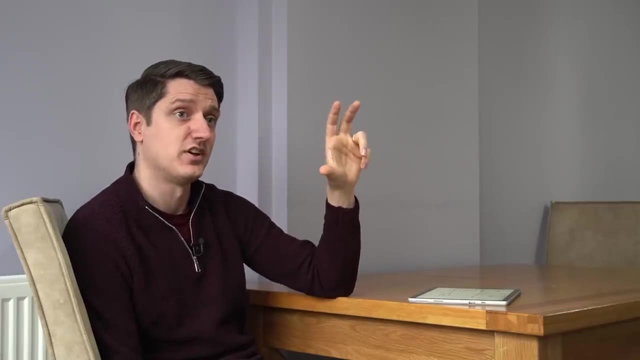 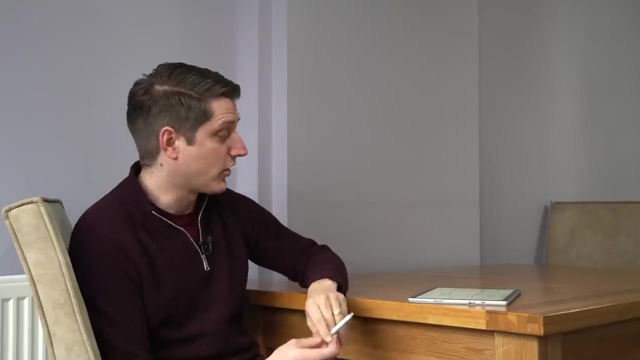 certificate with a um that has a public key on it and you will send a certificate verified message in tls 1.3, for example, which has a summary of some of the previous messages hashed, padded and encrypted using a private key right to verify. so you don't actually send the document because 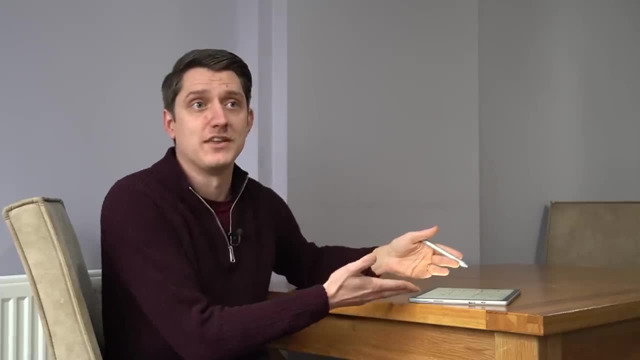 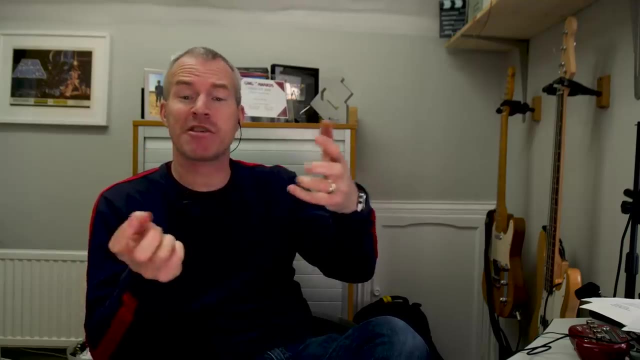 the document is the previous tls messages, right. so you know what that document is. we know what it is that we can, uh, we have to be checking against. basically, you're doing a um, a comparison right between what you've already received that you've then hashed and add padding to. 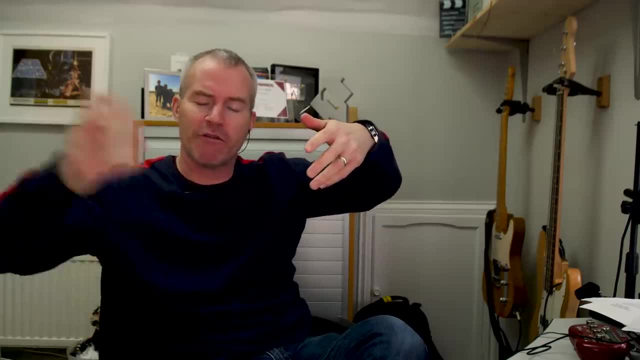 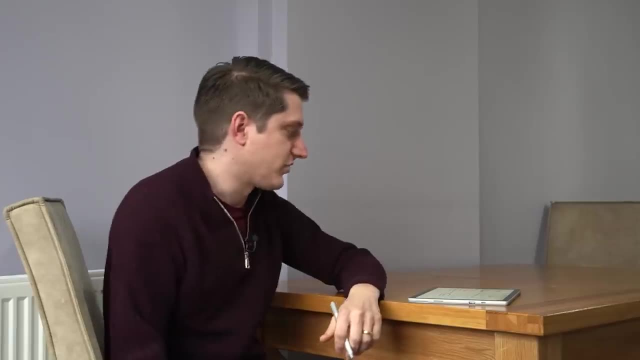 and then what you receive as the kind of authorization or confirmation that that should be the right thing. how do we we know what padding and stuff. is that like a system? is it like a set? that's a great question. yeah, so we would usually use something like the probabilistic signature. 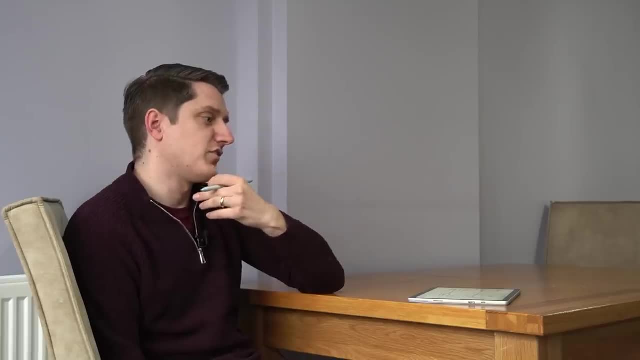 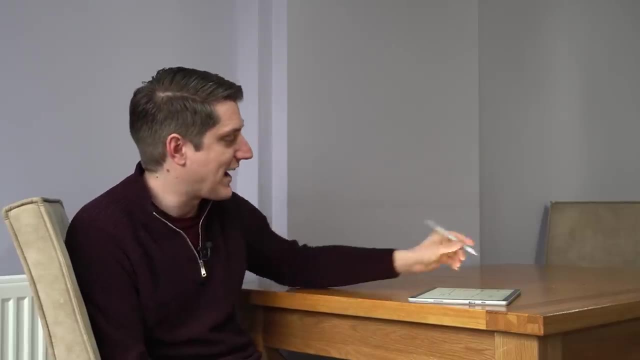 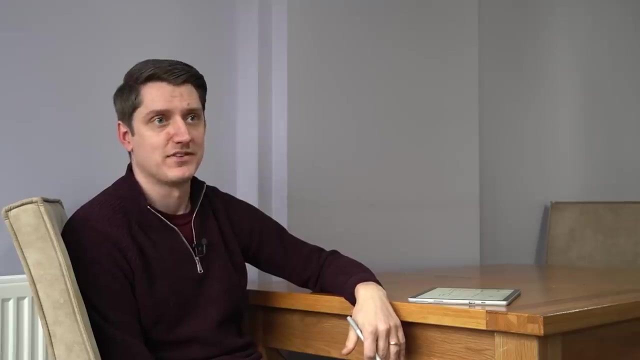 scheme for rsa right, and, and these introduce essentially a formal structure for doing this. they also tend to add something like a salt or a random number, which means that um messages encrypt differently each time. it's never a secret, it's just for it. it it helps with the implementation. 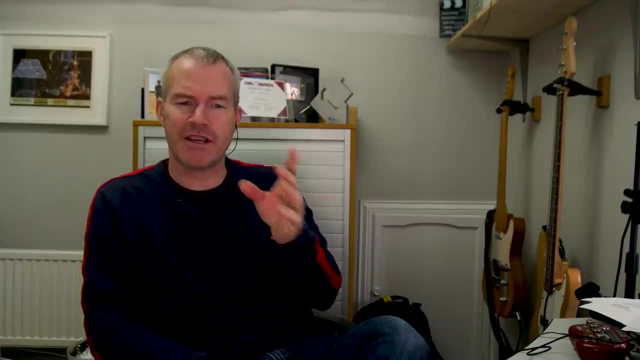 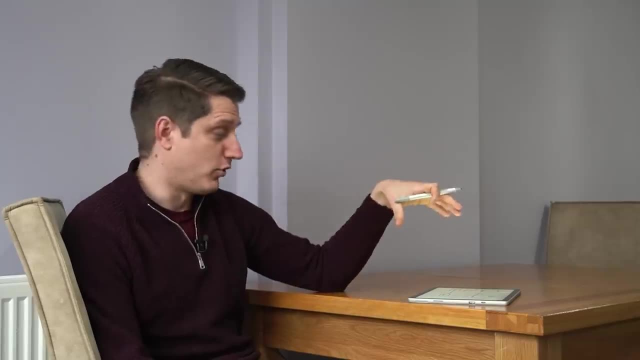 and the security. we're talking about any document here. this isn't the certificate that we sort of started talking about at the beginning, is it? it could be, it could be, and often it is. one of the primary roles for digital signatures is on the end of certificates, right as part of public key.